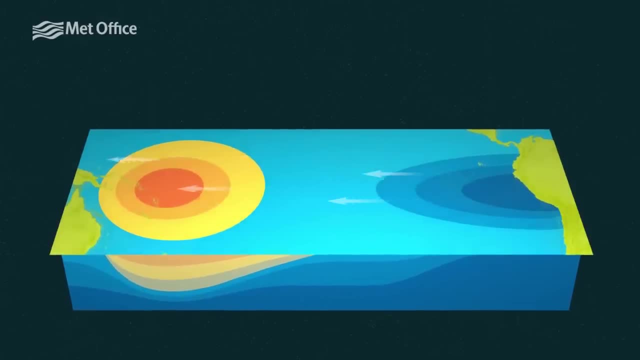 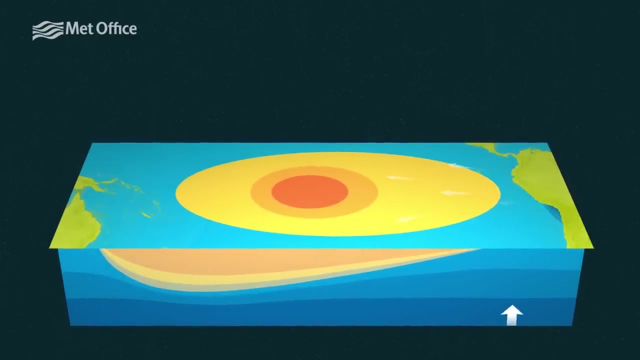 With weakened trade winds, there's less push of warm surface water to the western side of the ocean and less upwelling of cold water on the eastern side. This allows the usually colder parts of the ocean to warm, cancelling out the normal temperature difference. 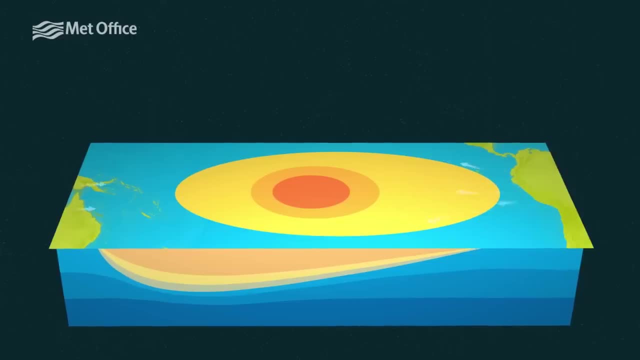 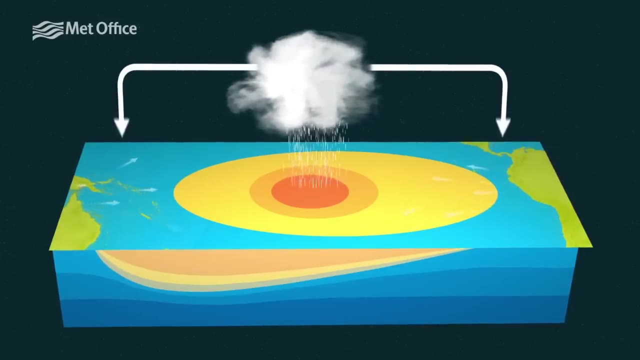 Because the area of warmest water moves, so does the associated wet and unsettled weather. unsettled weather: This changes rainfall patterns over the equatorial Pacific, as well as the large-scale wind patterns. It's this change in winds which has a knock-on effect changing. 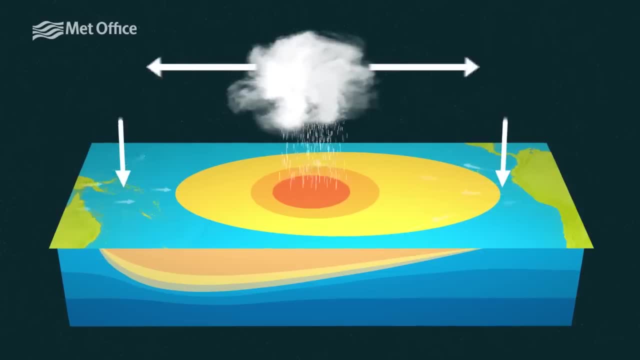 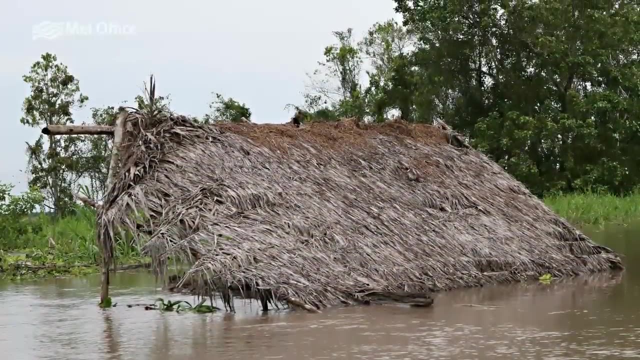 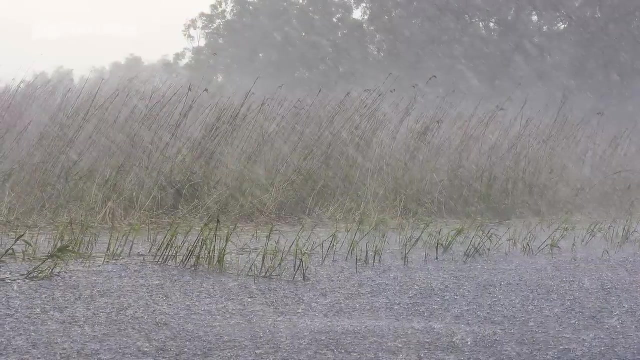 temperature and rainfall in locations around the world. The main impacts are around the tropics, where you see an increase in the risk of floods in Peru and droughts in Indonesia, India and parts of Brazil. But virtually wherever you are in the world, El Niño has the potential to affect you directly via the weather or 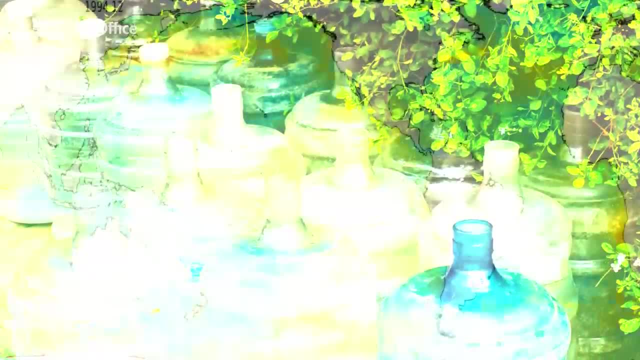 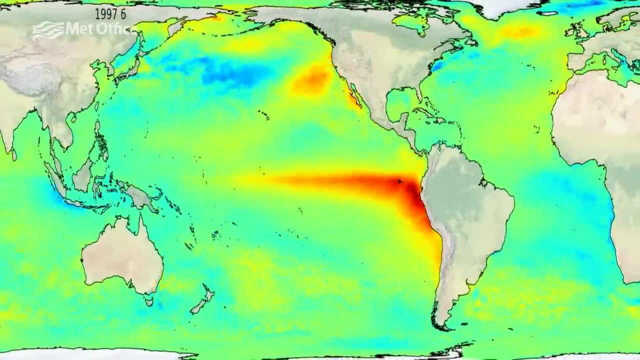 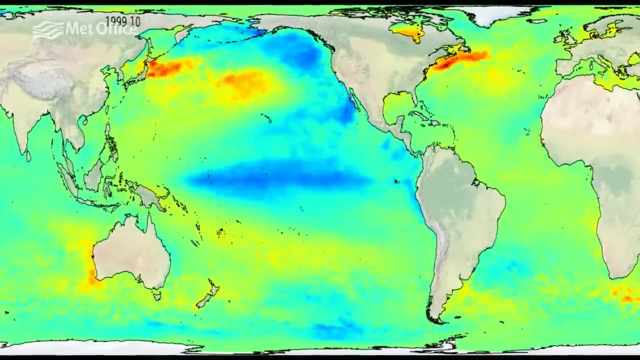 indirectly via socio-economic impacts. There's another impact from El Niño, which happens because of all the extra heat at the surface of the tropical Pacific. This releases vast amounts of energy into the atmosphere, which can temporarily push up global temperatures. This is why El Niño years often feature among 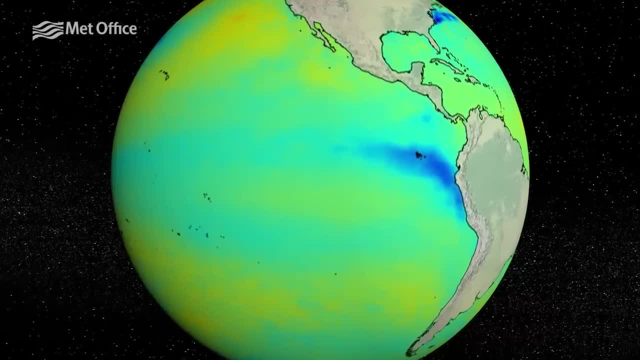 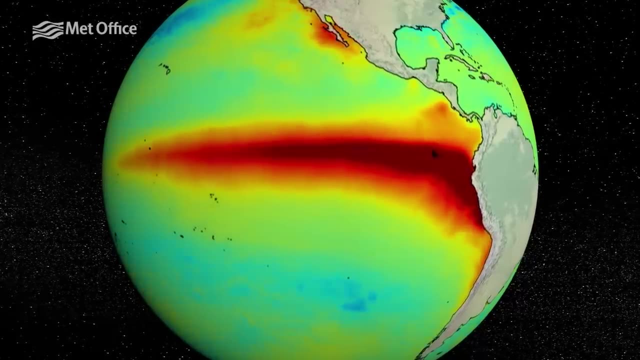 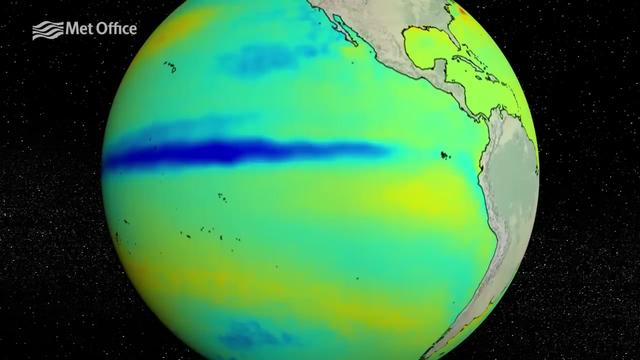 the warmest on record. Each El Niño event is different, so the global impacts can change. You can find out more about the differing impacts of El Niño on our website. El Niño peaks around Christmas time and lasts for several months. It can die back to neutral. 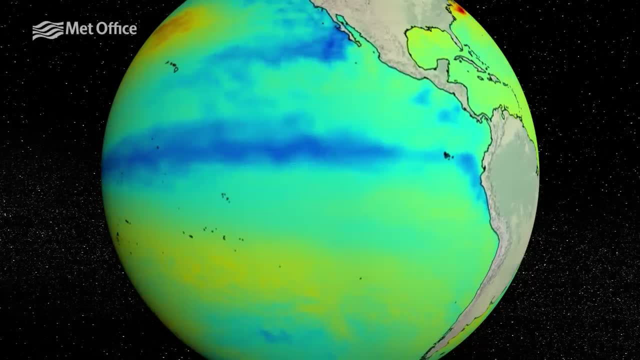 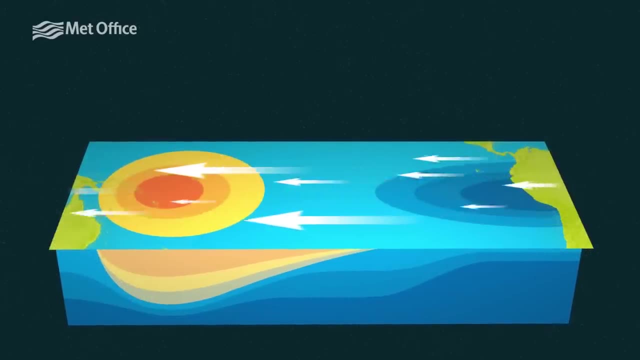 conditions, but sometimes reverses into La Niña. This is the flip side of the oscillation, which sees a strengthening of the normal trade winds. This pushes the warmest water down to the upper part of the ocean andistäces a strengthening of the normal trade winds. 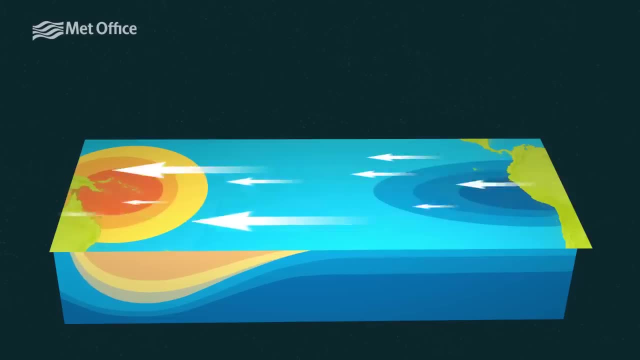 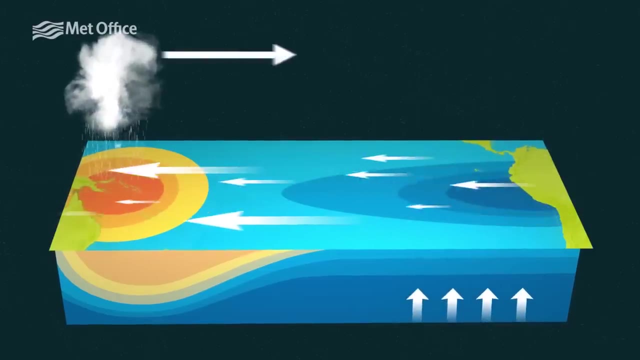 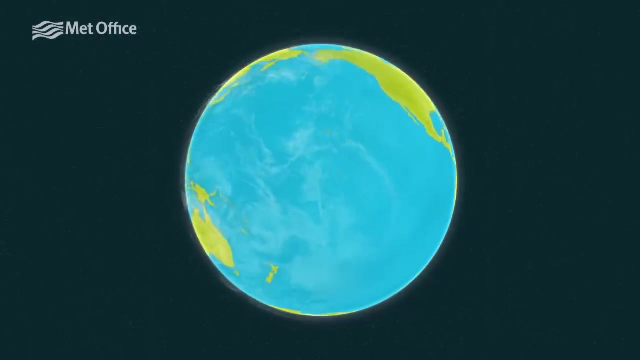 to the far western part of the tropical Pacific and increases the upwelling of cold water. in the east, This cooler water extends out from the coast of the Americas towards the central part of the ocean. La Niña also impacts global weather and tends to have opposite. 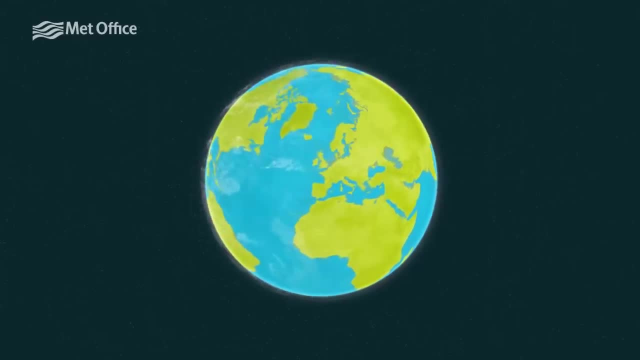 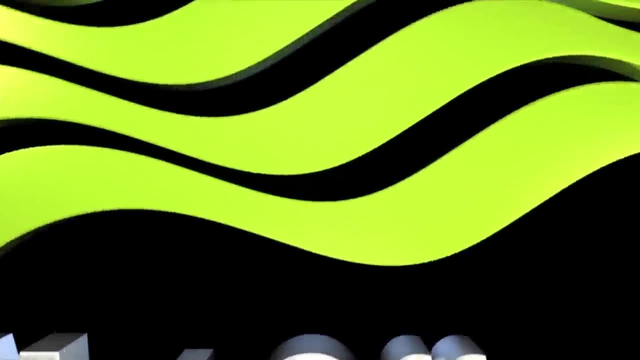 effects to El Niño. You can also see more about La Niña and its impacts on our website. Subtitles by the Amaraorg community.